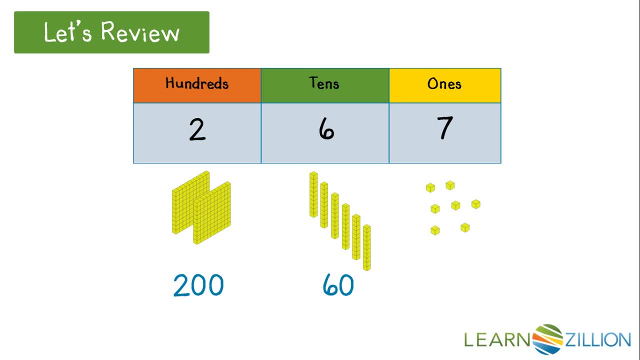 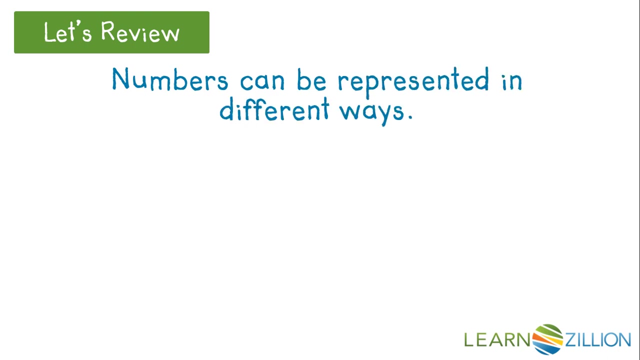 The 6 is in the tens and has a value of 60, and the 7 has a value of 7 ones. Each digit has a specific value based on its place within a number. It is also important to remember that numbers can be represented in different ways. 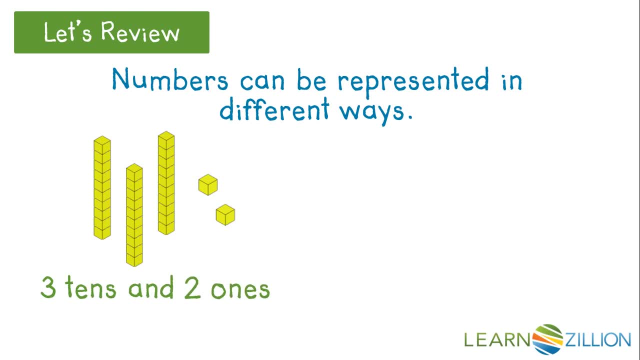 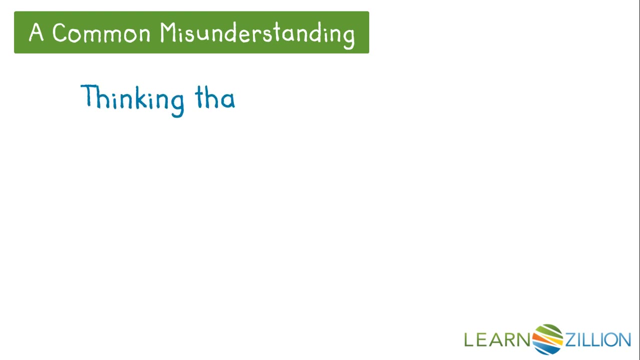 Three tens and two ones, as well as two tens and 12 ones. both represent the same amount. Each picture shows the amount of 32.. A common misunderstanding that many students make is thinking that the 4 and 46 has a value of 4 instead of 40. if we look at the digits in 46, we can see that the 4 is in. 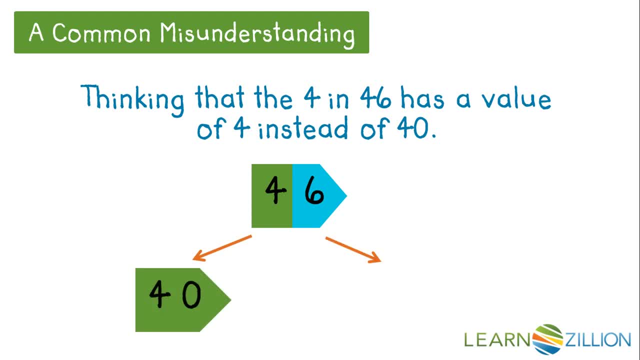 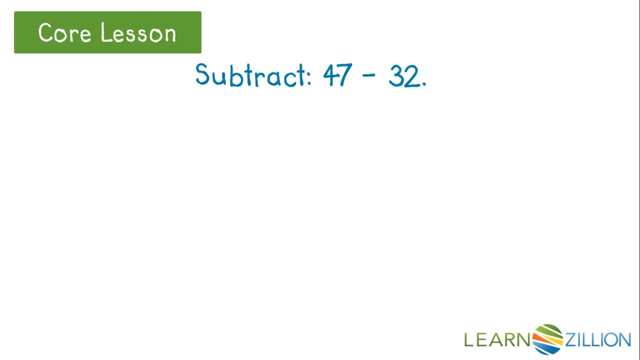 the tens place. therefore, the 4 has a value of 40, not just 4. now let's subtract 32 from 47. first I need to think about the value of each digit. the 4 and 47 has a value of 40 or 4 tens and the. 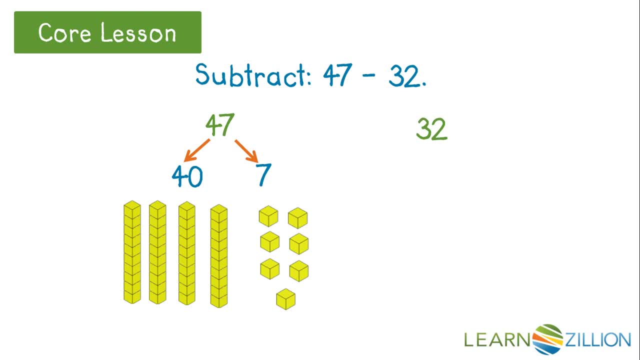 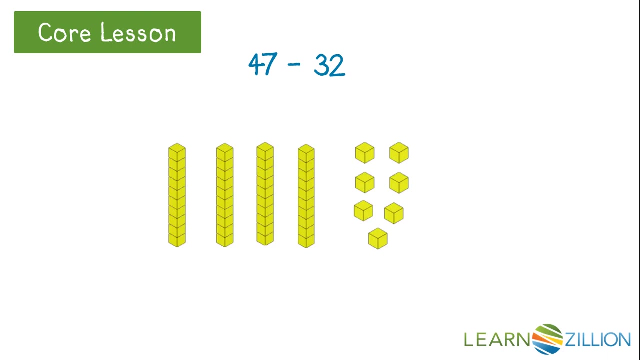 7 has a value of 7 ones, the 3 in 32 has a value of 30 or 3 tens and the 2 has a value of 2 once. so if we start with 47 and take away 32, I can see that 47 is. 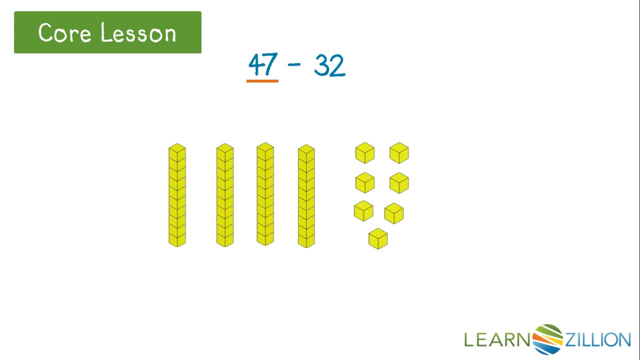 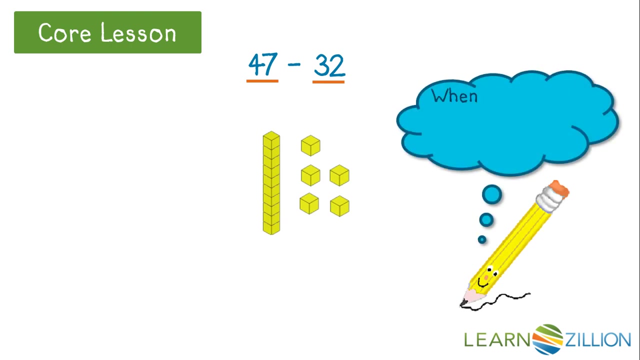 made up of four tens and seven ones. I need to take away three tens and two ones. when I take away 32 from 47, I end up with 15. 47 minus 32 equals 15. now let's subtract 54 minus 26. again, I need: 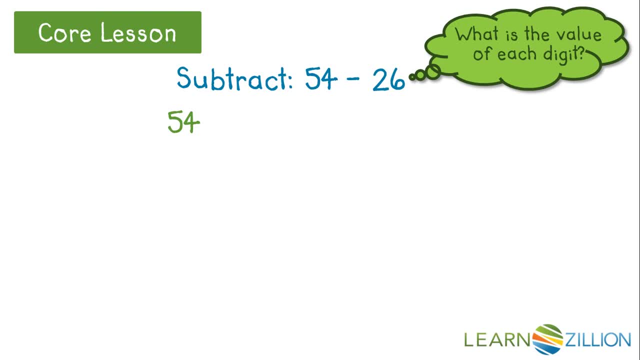 to think about the value of each digit. the 5 and 54 has a value of 50 or 5 tens, and the 4 has a value of 4 ones. the 2 and 26 has a value of 20 or 2 tens, and